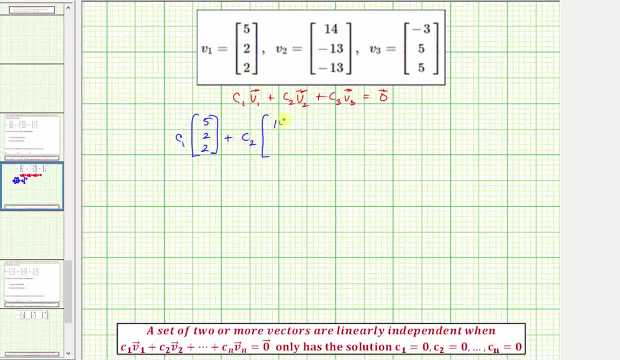 plus C sub two times V sub two plus C sub three times V sub three equals a zero vector. Let's write this as an augmented matrix, and then we're going to reduce our echelon form, So we'll have a three by four augmented matrix. 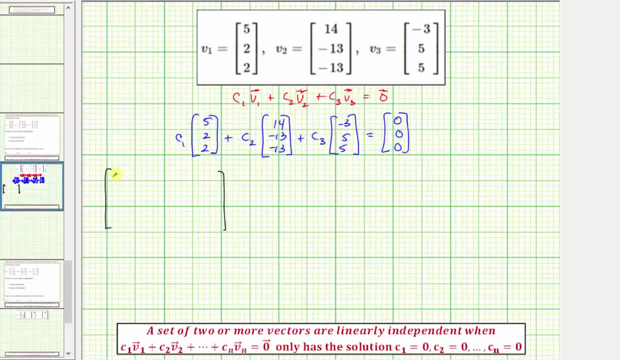 where the first row would be five 14, negative three- zero. The second row would be two negative 13,, five zero And the third row would also be two negative 13,, five zero. So notice right away row two and row three. 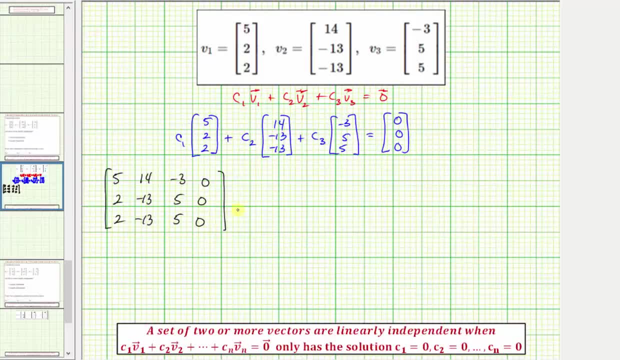 are the same. So let's obtain a row of zeroes by replacing row three with negative one times row three plus row two. Let's also get a leading entry of one in the first row. Notice that negative two times two plus five would be one. 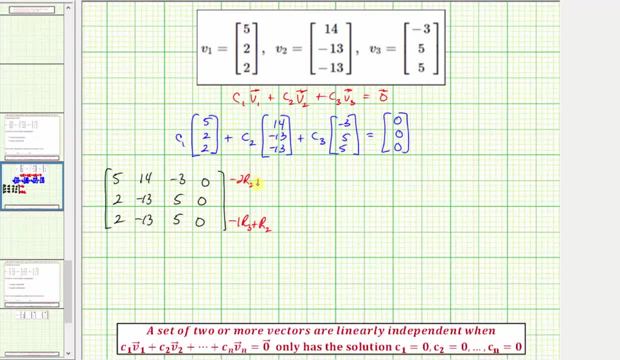 Let's replace row one with negative two times row two plus row one. So in the first row we'd have negative two times two plus five, that's one, And then we'd have negative two times negative 13,, that's 26, plus 14,, that's 40.. 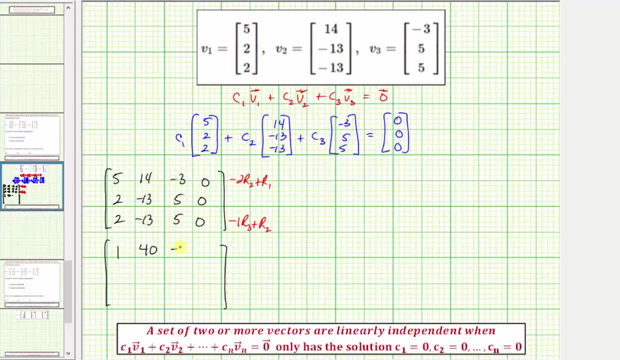 Negative two times five, that's negative 10, plus negative three, that's negative 13,. and then we'd have zero. Second row stays the same. So because we have a row of zeroes we already know we're going to have 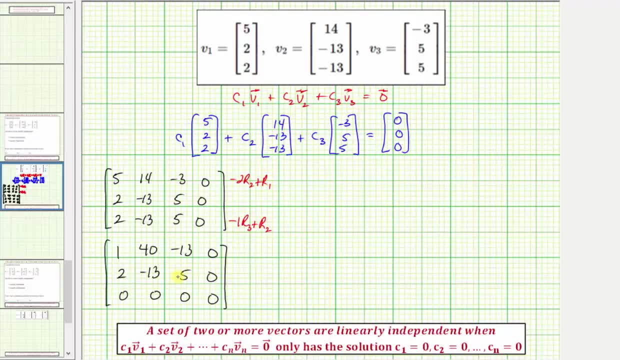 an infinite number of solutions and therefore the vectors are linearly dependent. But we still need to express the relationship between C sub one, C sub two and C sub three in order to write vector V sub three as a linear combination of V sub one and V sub two. 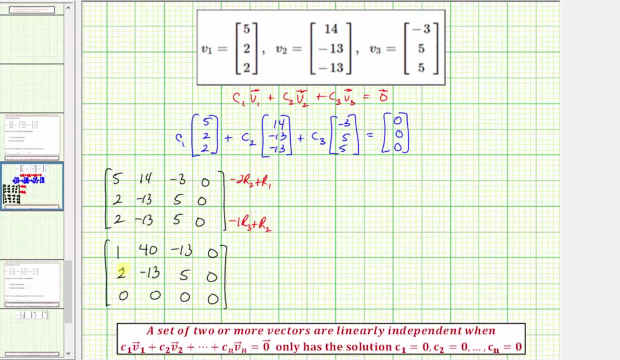 So the next step: let's get a zero here by replacing row two with negative, two times row one plus row two, And we'll keep row one and row two the same for right now. So the first row stays the same, The last row stays the same. 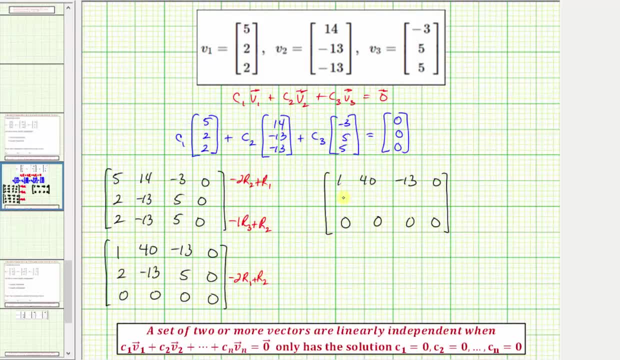 And now for row two. we have negative two times one plus two, that's zero. Negative two times 40 is negative 80, plus negative 13,, that's negative 93.. Negative two times 13 is 26,, plus five is 31,. 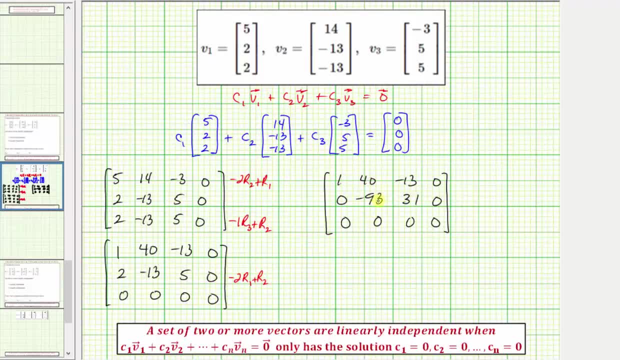 and then we have zero. Now let's get a leading entry here of one by replacing row two with negative one over 93 times row two. So row one and row three stay the same, And then for row two we'd have zero one. 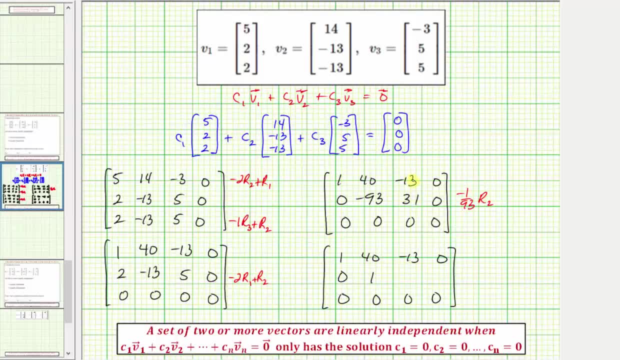 and then negative one over 93 times 31 actually simplifies to negative 1, 3rd, And then we have zero Again. we multiply negative one over 93 times 31.. We get 31 over negative 93. But 93 is equal to three times 31.. 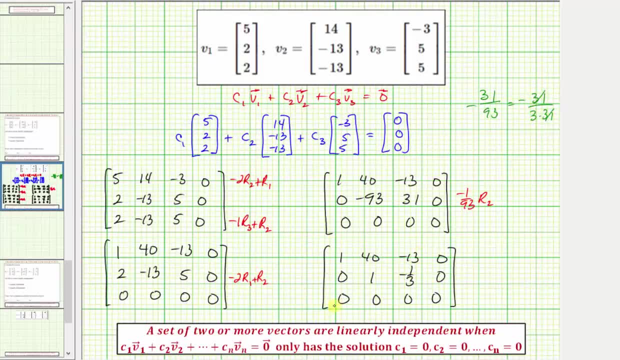 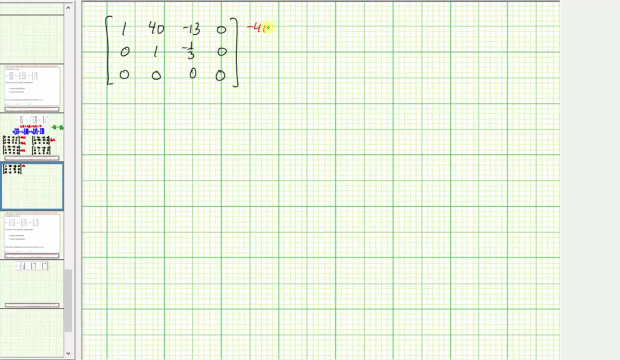 31, simplify out giving us negative 1- 3rd, Negative 1- 3rd. Let's continue on the next slide. For our last step, let's get a zero here by replacing row one with negative 40 times row two plus row one. 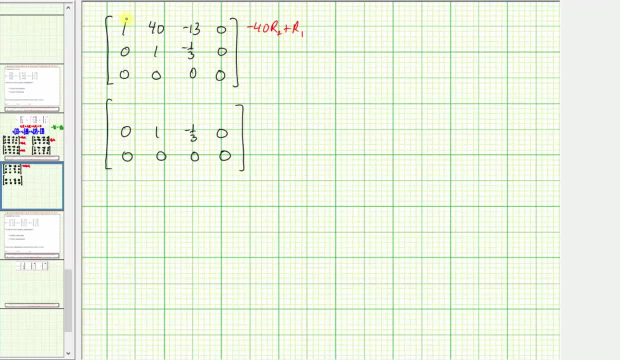 So the second and third rows stay the same. And now for row one, we'll have negative 40 times zero plus one. that's one Negative 40 times one plus 40, that's zero Negative 40 times negative. 1- 3rd, that's 40 3rds. 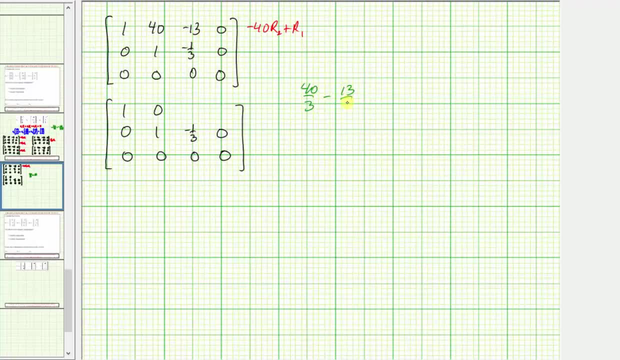 And then plus negative 13, or minus 13 over one common denominator of three. So our denominator is three. The numerator is 40 minus 39, which is one. So we have 1, 3rd and then zero. So now the augmented matrix is in reducible echelon form. 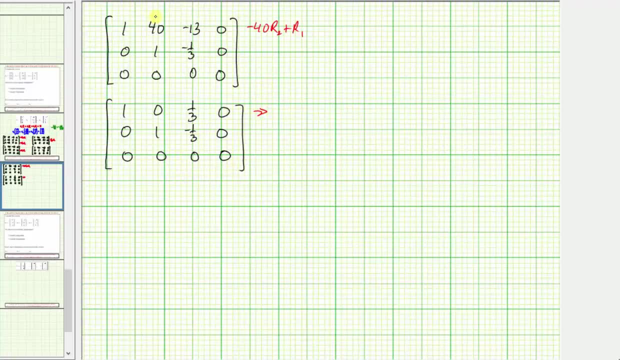 We already know there's a non-zero solution. Notice: the first row tells us that C sub one plus zero, C sub two plus 1. 3rd C sub three equals zero. And the second row tells us that one C sub two or C sub two minus 1. 3rd C sub three equals zero. 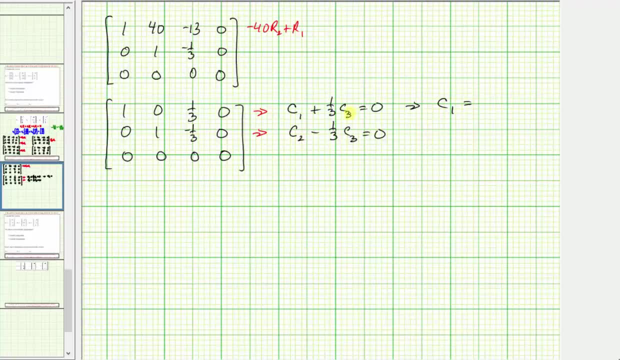 So here we know that C sub one must equal negative 1- 3rd C sub three, And we know that C sub two must equal positive 1- 3rd C sub three. So we can use these relationships to express vector V sub three as a whole. 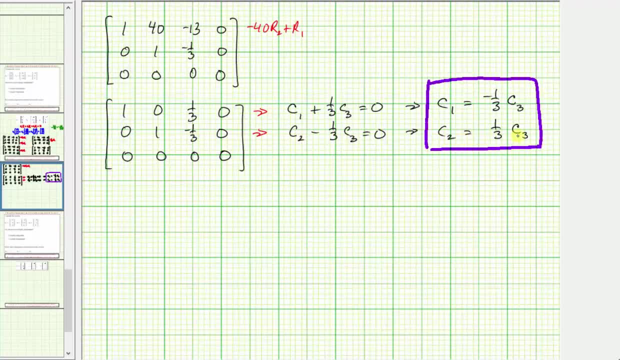 As a linear combination of vector V sub one and V sub two. Remember our vector equation was: C sub one times vector V sub one plus C sub two times vector V sub two plus C sub three times vector V sub three equals the zero vector. So if we solve this for C sub three times vector V sub three, 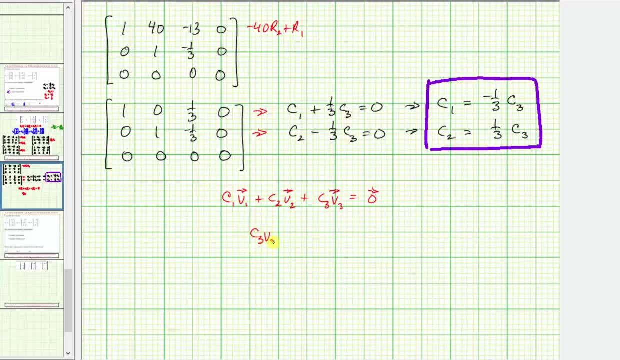 we'd have C sub three times vector V sub three, equals. we can leave off the zero vector and this would be equal to negative c sub one times vector v sub one minus c sub two times vector v sub two. So if we want to write v sub three, 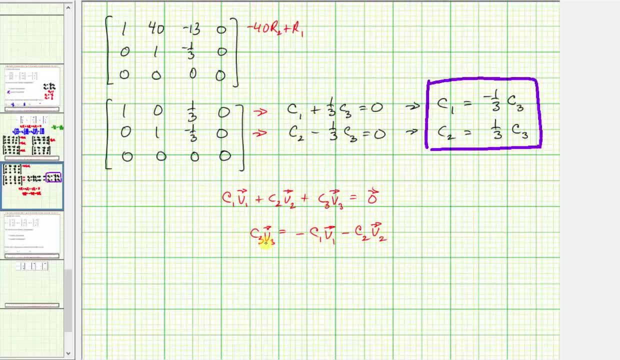 as a linear combination of v sub one and v sub two. notice how c sub three would have to be equal to one And if we know c sub three equals one, we have the equations here. we need to find c sub one and c sub two. 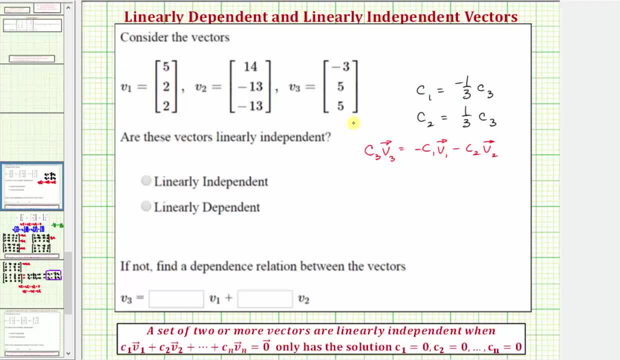 So, going back to our first slide, we now know the three vectors are linearly dependent, because the solution to our vector equation was not just c sub one, c sub two and c sub three equals zero. And again now to express vector v sub three. 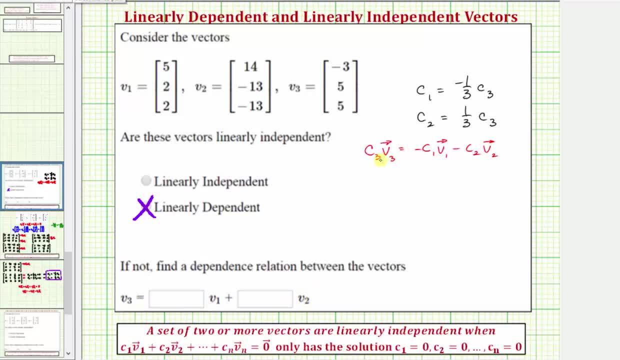 as a linear combination of v sub one and v sub two. if we want v sub three here, notice that c sub three is equal to one. So if c sub three is equal to one, notice how this tells us that c sub one is equal to negative. 1. 3rd. 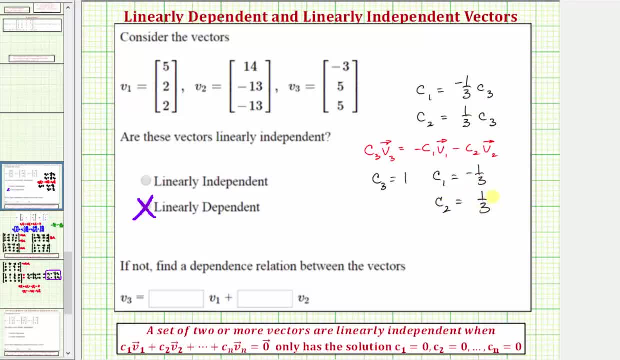 and c sub two is equal to positive 1- 3rd. So we need to be careful here, because notice how the right side of this equation is negative: c sub one times vector v sub one, minus c sub two times vector v sub two. So because c sub one is negative 1- 3rd. 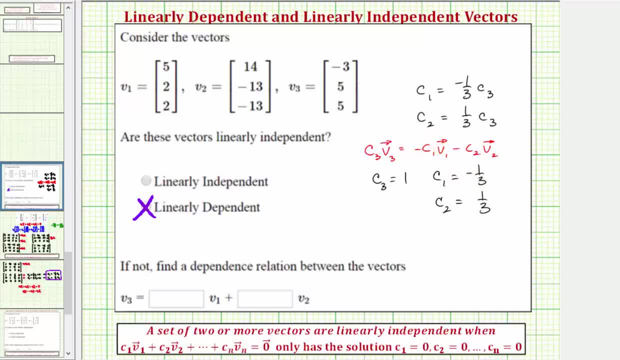 the scalar here is going to be positive: 1, 3rd. So v sub three equals 1, 3rd times v sub one. And then, because we have minus c sub two times vector, v sub two and c sub two is positive 1, 3rd. 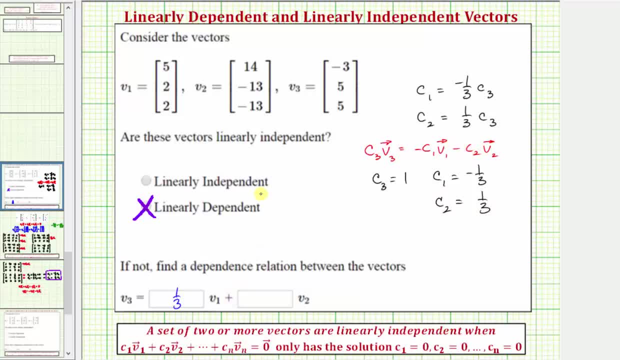 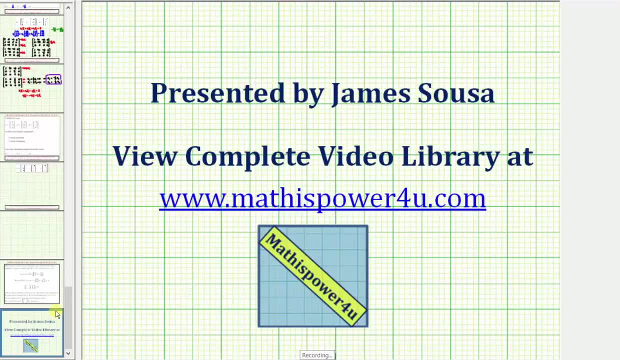 this would be minus 1 3rd. Because we have a plus sign here, the scalar here is going to be negative 1 3rd. I hope you found this helpful.